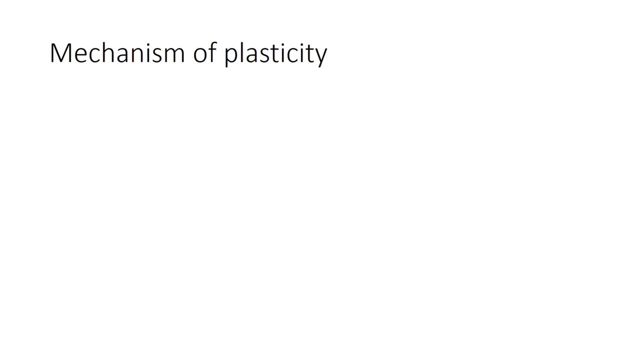 Let me start with the mechanism of plasticity. Metal plasticity is due to shear, whereas in rock or soil plasticity it also depends on pressure. Let's focus on the metal plasticity here. Sliding of atomic planes over one another at the molecular level causes plastic deformation at the continuum scale. 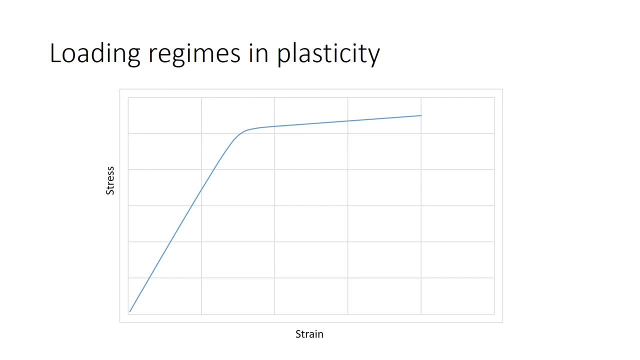 This is a uniaxial stress-strain curve for general ductile material. When you load the material beyond the yield stress, you get plastic deformation. There are 2 regimes with respect to the yield. The 1st one is the elastic regime. 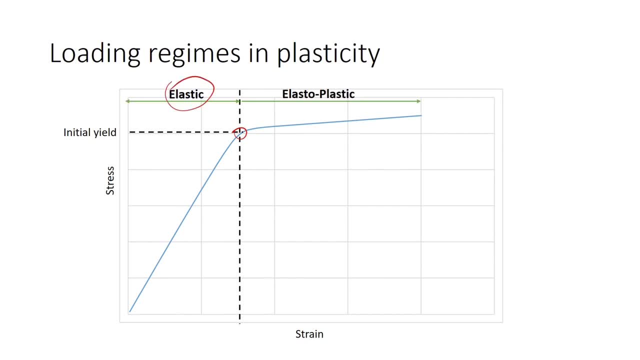 It is well known that the loading and unloading curves follow the same path. The 2nd one is the elastoplastic regime. In real materials, beyond initial yield there will be both elastic and duplication. Then it comes out to the rough surface and it is theutive겨 Ganga zone. 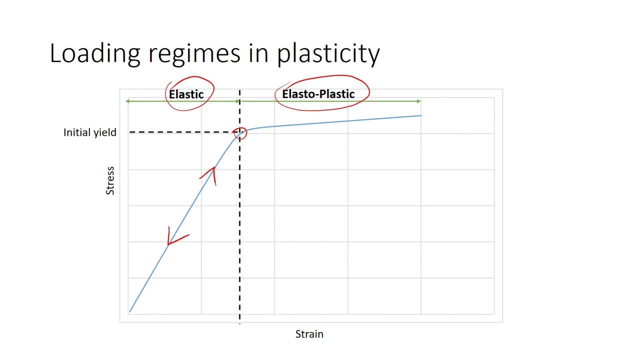 So in the Lisa- Vadakha level, plastic seasoning technology is used for the use of plastic deformation. It is mena, Pedan, Say you like it or you ignorant. Describe your product Close, Describe it. and plastic deformation In elastoplastic regime. the loading and unloading paths are different. 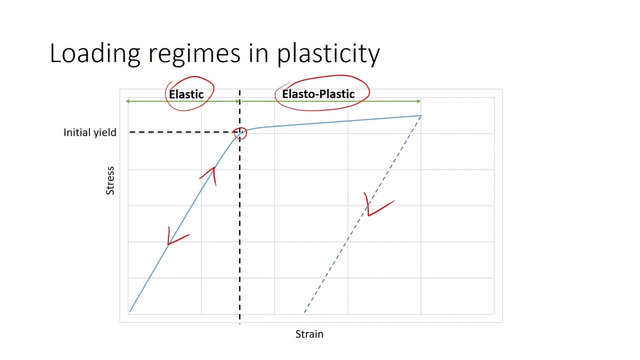 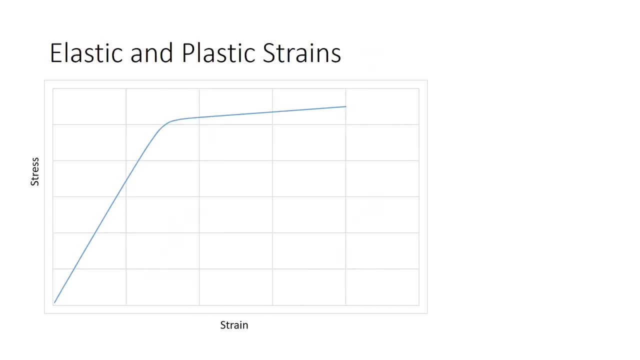 The unloading path is elastic and will be parallel to this line. Let's extend this argument to the strains. Let's say we loaded the material to a point A in the elastoplastic region. Strain at A will be the sum of both elastic and plastic strains. Let me explain how to obtain them. 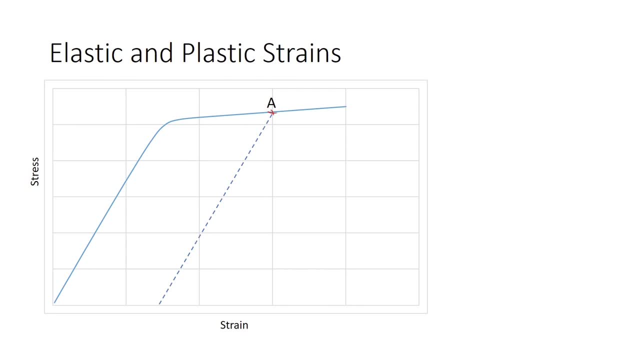 Let's do an imaginary unloading from A- This was our initial strain, epsilon A- and after unloading we are left with this much amount of strain. In other words, we have recovered this much amount of strain upon unloading and, by definition, it is the elastic portion of the strain. This portion. 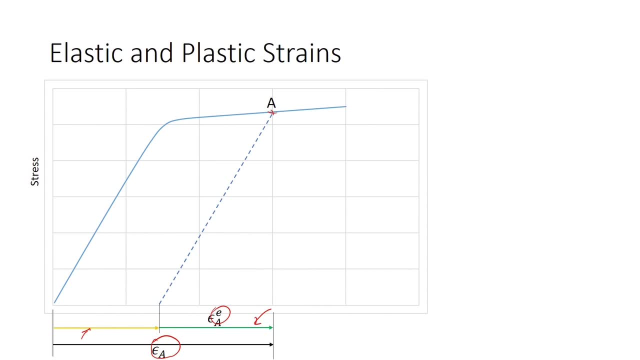 here the yellow line is the permanent deformation after unloading, and this is the plastic portion of strain. So we have epsilon A as a sum of elastic and plastic strains. This equation is known as the additive decomposition of strain, and note that it is only valid for small deformations With regard to stress there is. 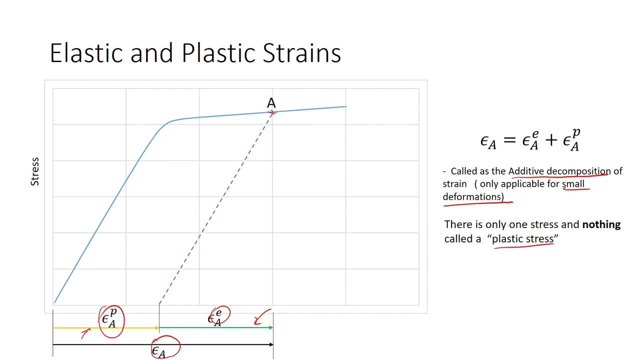 only one stress and that is stress, and there is nothing called as a plastic stress. This is a common misconception in the community. Let's consider points A, B and C along the unloading path. If you decompose the strain, you will find that all the points A, B and C have the same amount. 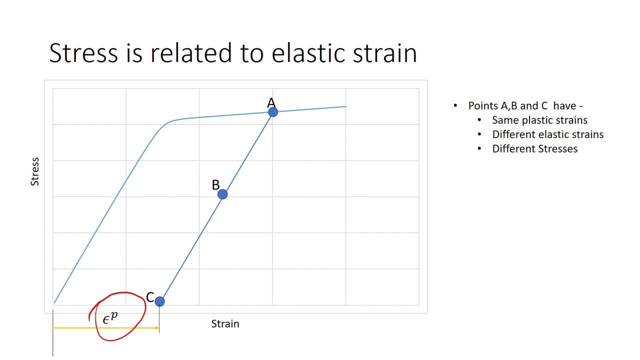 of plastic strain. as shown and from the figure it can also be seen that all A, B, C- have different stresses, Although the stresses change but the plastic strain remains constant. So the stresses aren't directly related to the plastic strains, or in other words the plastic strains. 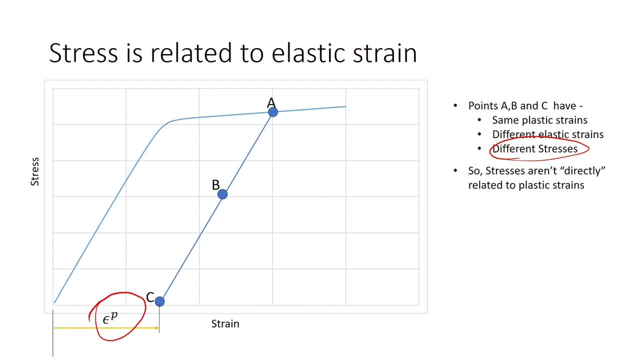 do not induce any stress. The stresses are related to elastic strains. For example, the stress at B is equal to the Young's modulus times the elastic strain at B. Now let's measure the strength of the material and while we're engineering, counter expects the 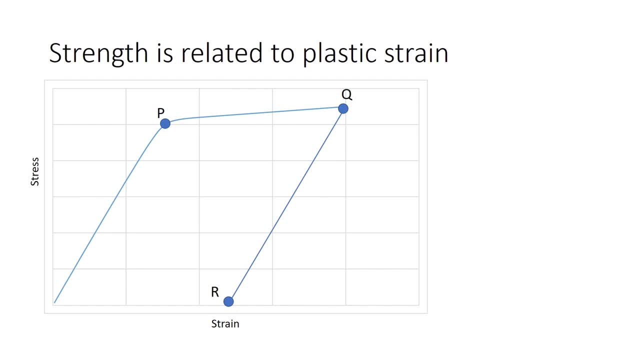 stress of this material means that it will be strong. Hence we may want to know what the stress on this material is. What does the plastic strain contribute to? Plastic stress contributes to the strength. Let's load the material till Q and then unload it to R and 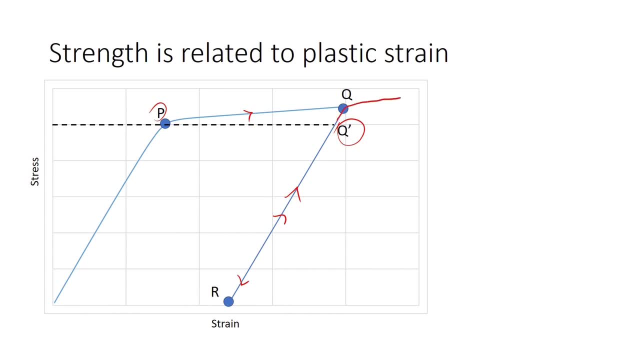 note that P is our initial yield. Now let's reload the material from R towards Q. It reduces the pressure which could be related to the plastic strain, epsilon p. when a material gains strength, it is known as strain hardening, and when it loses strength with plastic strain, it is known as. 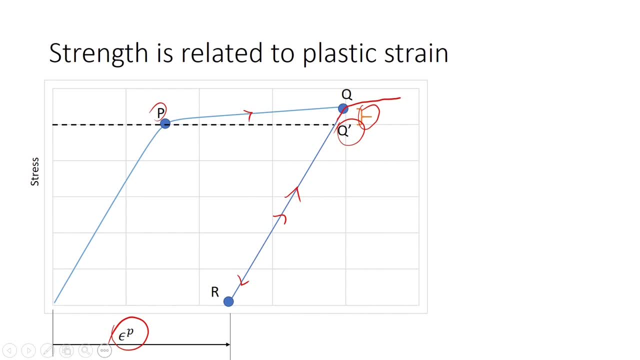 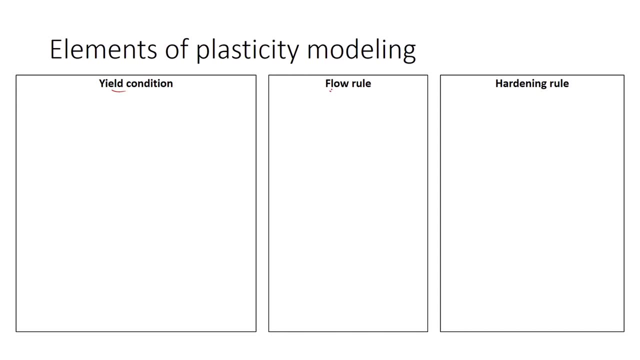 strain softening. with all that background, let's see how to model plasticity. there are three elements to plasticity modeling. they are the yield condition, the flow rule and the hardening rule. the yield condition is regarding the question: at what combination of stresses does a material yield? 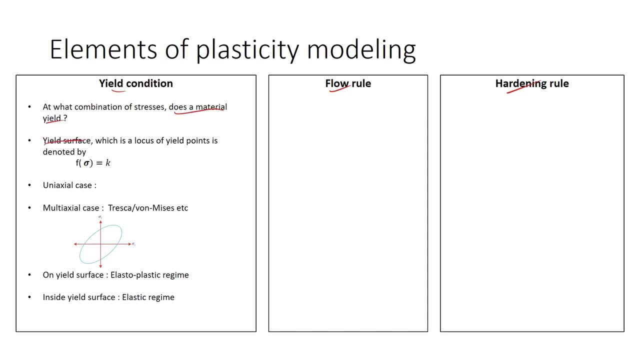 it is represented by the yield surface and it is denoted by the equation function of stress tensor equal to constant. let me give a couple of examples in this. for the uniaxial case, the yield equation is just sigma 1, equal to sigma y. for the multi-axial cases, things are a bit complicated. 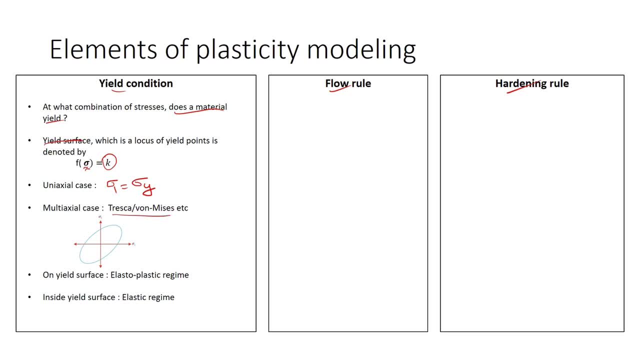 and tresca and von mises yield surfaces are the well-known ones. i have shown here the von mises yield surface, which is an ellipse in the principal stress domain. the stress state is on the surface. then it is in the elastoplastic regime if the stress state is. 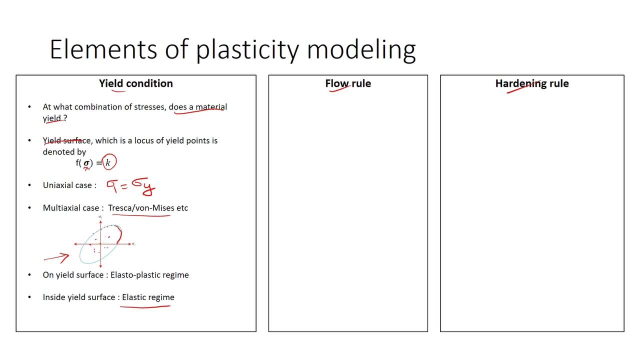 inside the surface, then it is in the elastic regime. note that the stress state can never go beyond the yield surface. the second one is the flow rule, which gives a mathematical description of how a material flows beyond the initial yield. it is roughly a relation between plastic strain.